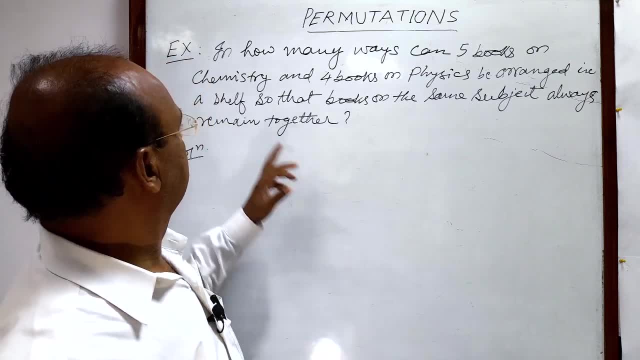 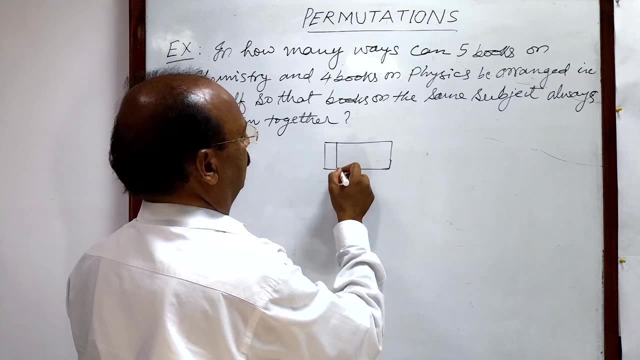 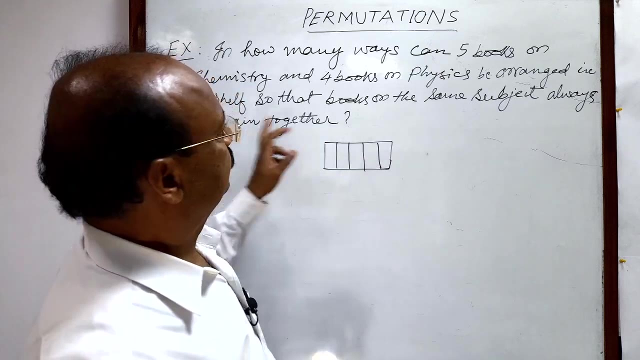 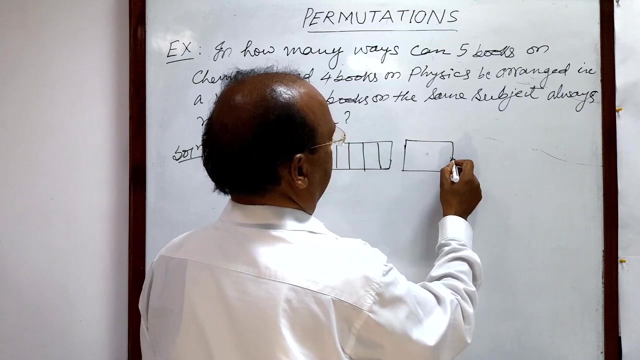 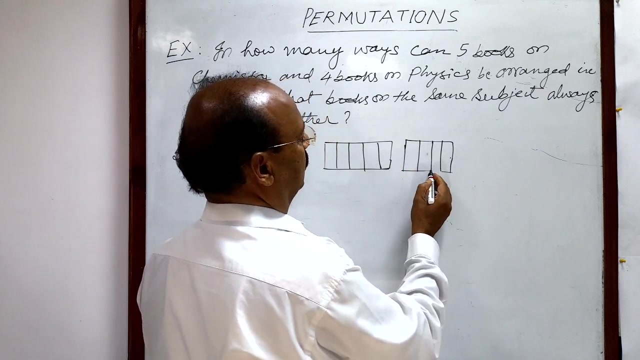 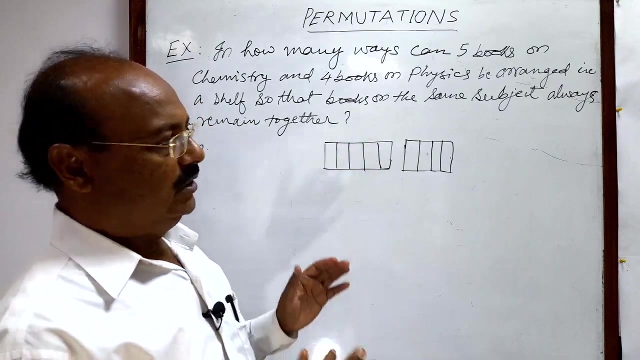 Let us make it clear. Five books of chemistry. Okay, suppose we are having here five books of chemistry: One, two, three, four. These are five books of chemistry, Five books on chemistry and four books on physics. Okay, and four books on physics- One, two, three, four books- Okay, these are four books on physics, And we have to keep these books in a self so that books of the same subject always remain together. 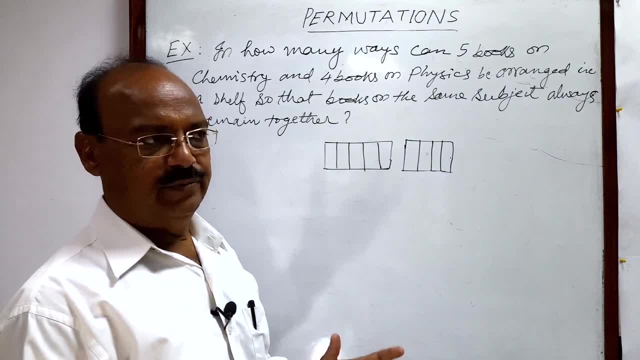 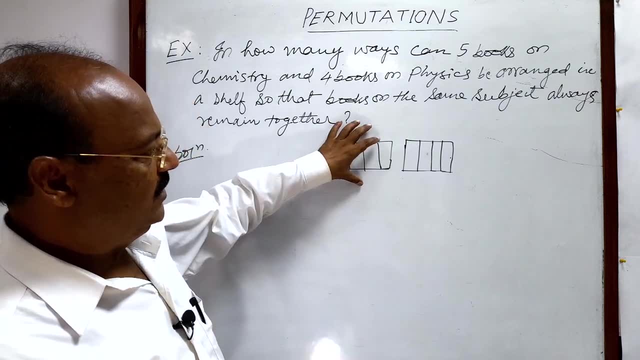 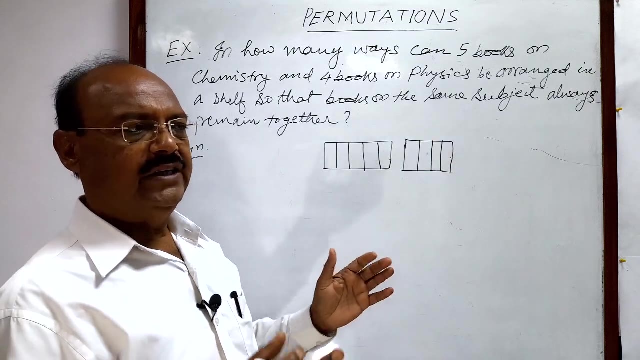 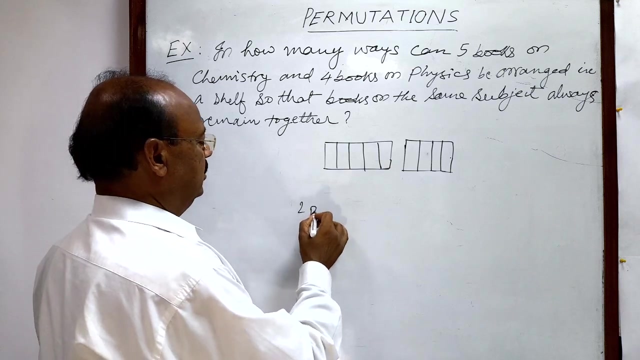 So what are the different options? What are the different options of arrangement? The total number of arrangements will be our answer. So, first of all, one set of chemistry book and one set of physics book can be taken as two objects and can be arranged in two different ways, in 2P2 ways. 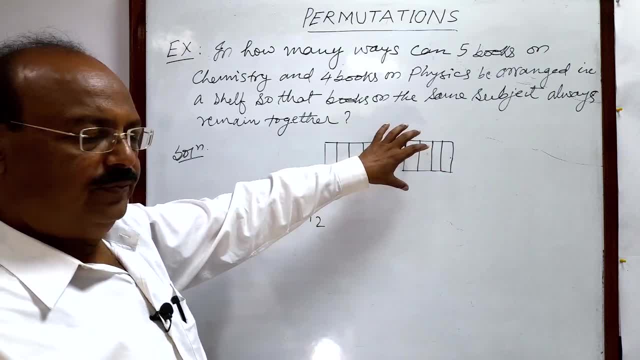 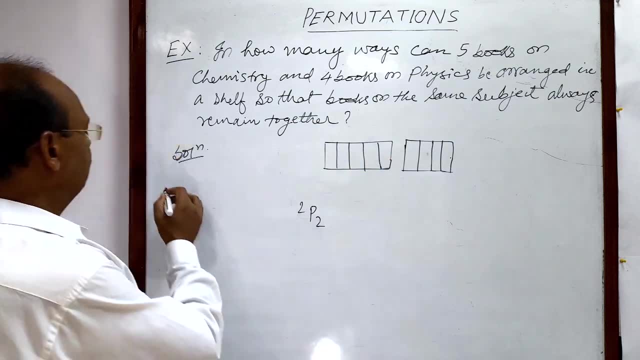 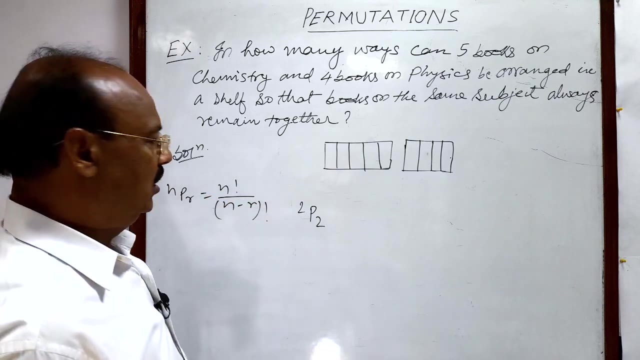 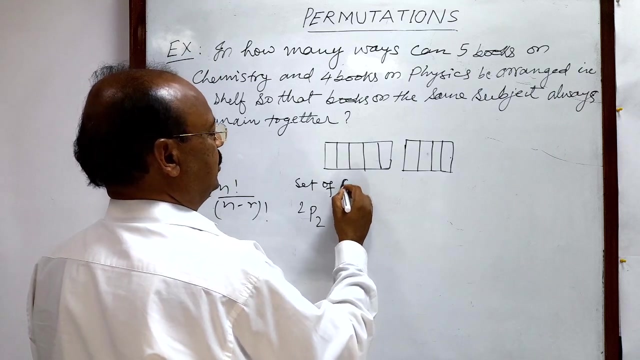 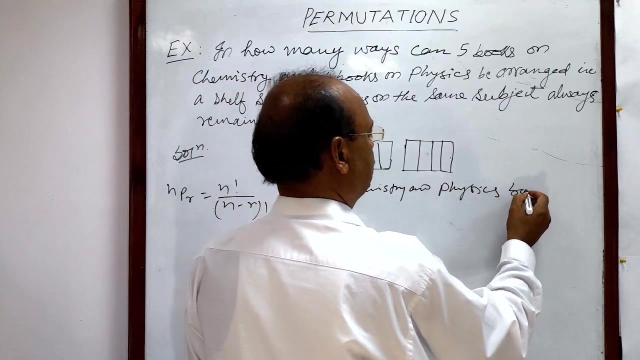 Total number of objects is two and options are two Objects taken at a time. two means two sets, Okay, and we have to use the formula here: NPR is equal to N factorial by N minus R whole factorial. So here set of chemistry and physics books. 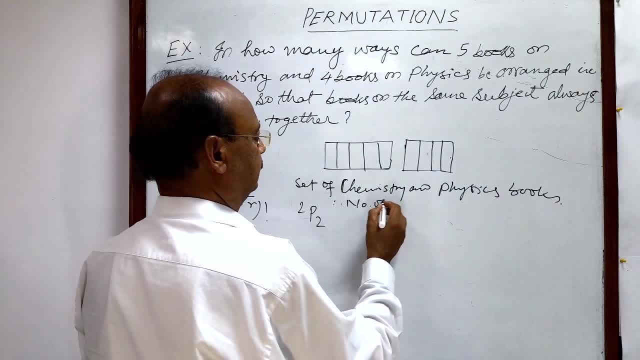 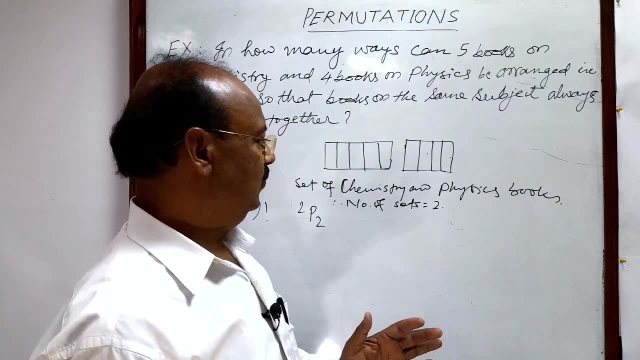 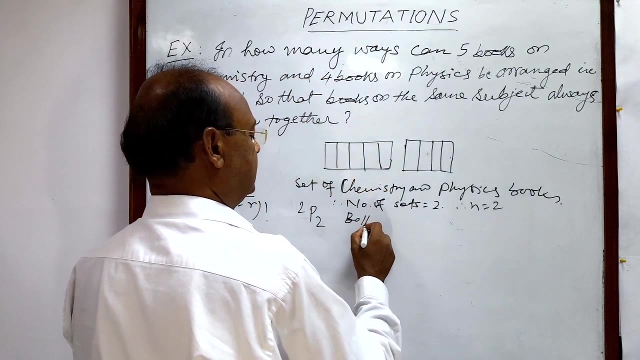 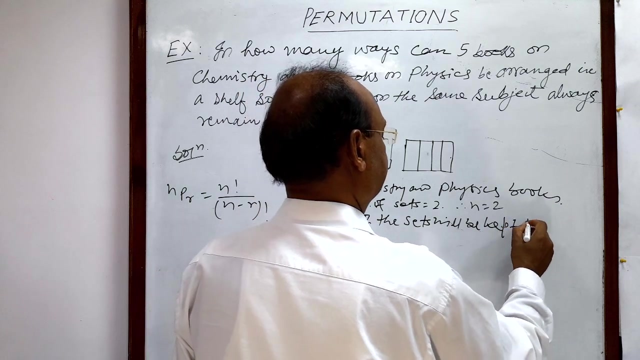 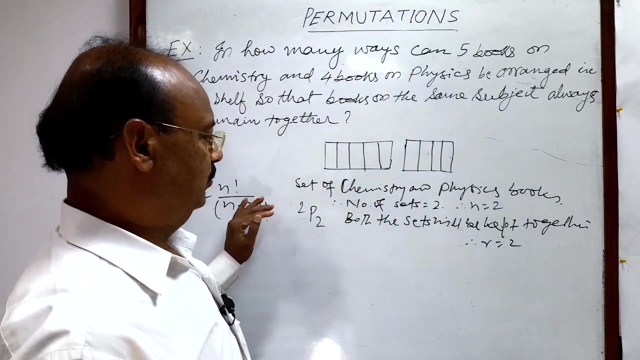 So, therefore, number of sets N is equal to 2 and both the sets have to be kept together. So therefore, N is equal to 2 and both the sets will be kept together. Therefore, R is equal to 2 as per permutation process. 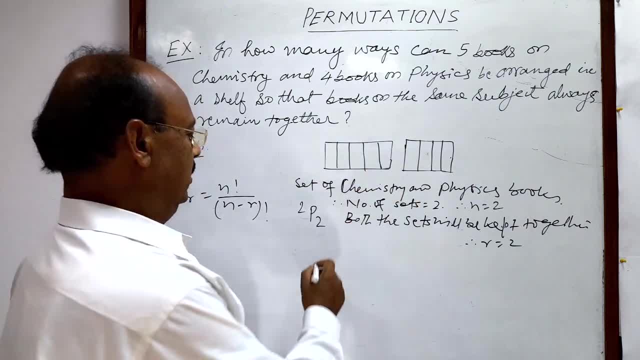 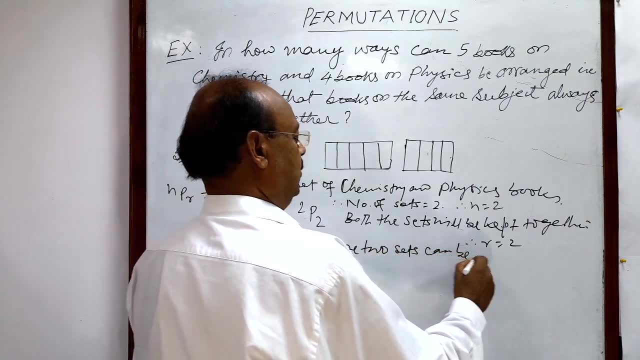 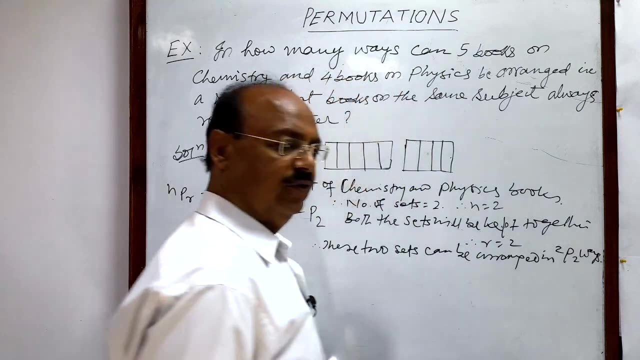 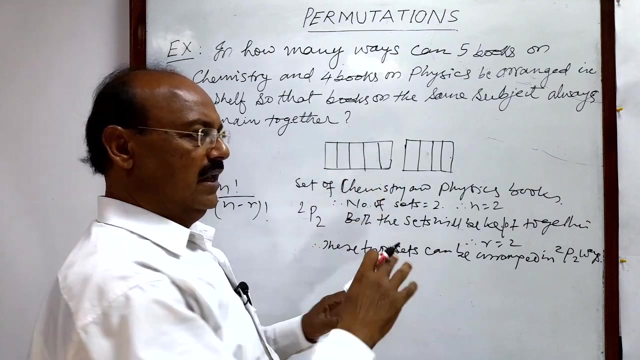 So these two sets can be arranged in. therefore these two sets can be arranged in 2P2 ways. Fine, One step, Now another step. These five books can be arranged among themselves in how many ways? Here N is equal to. 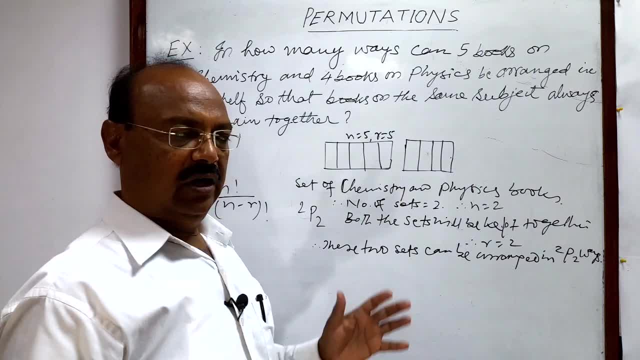 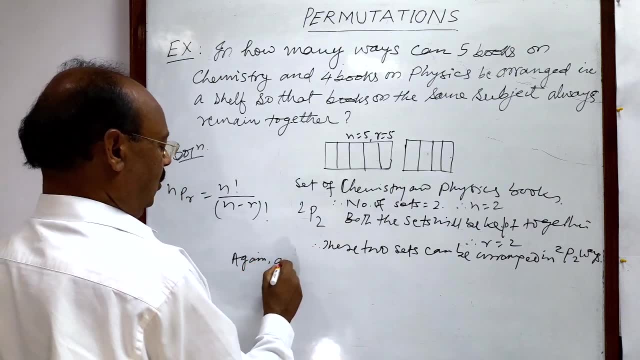 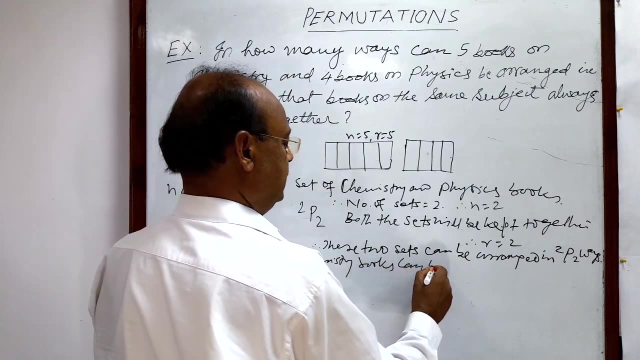 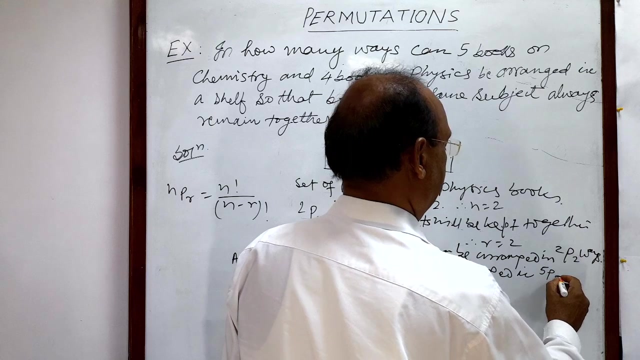 Five, Five And R is equal to five, because all the chemistry books have to be taken together. Again, all chemistry books can be arranged in five P5 ways. Okay, Total number of books is five. All have to be taken together. 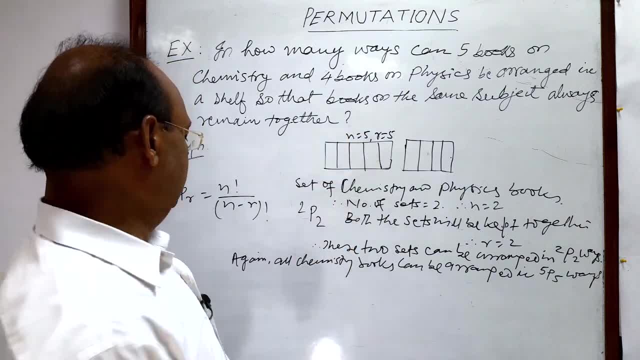 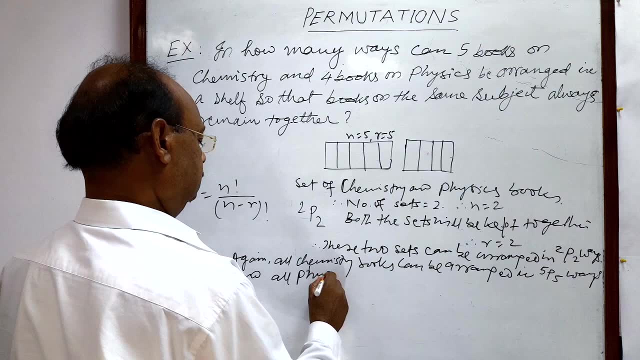 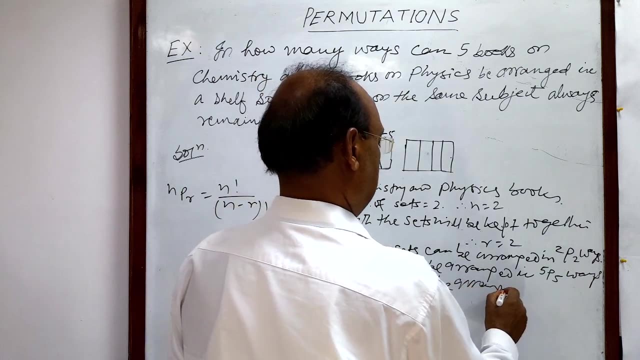 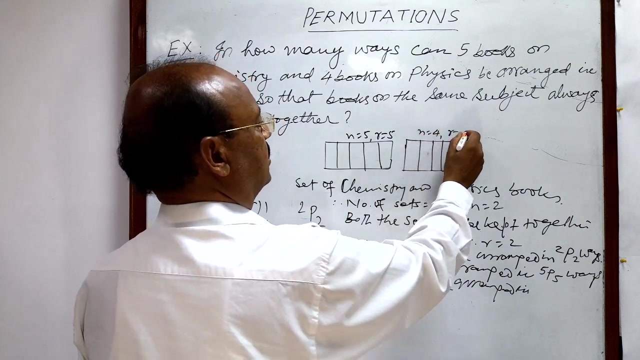 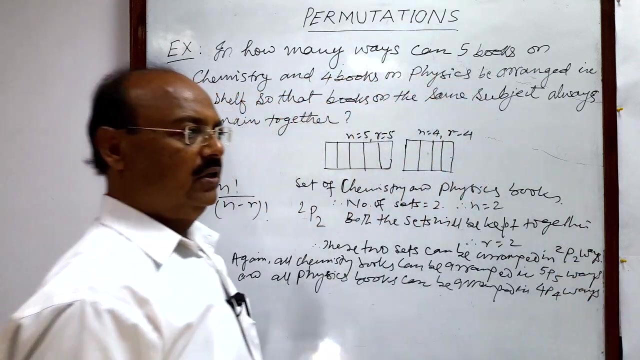 taken. all have to be arranged, so r is five. similarly, and all physics books, all physics books can be arranged in. total number of books is four here. so in this case n is equal to four and r is equal to four. so total number of ways is four, p four, which okay. so all the 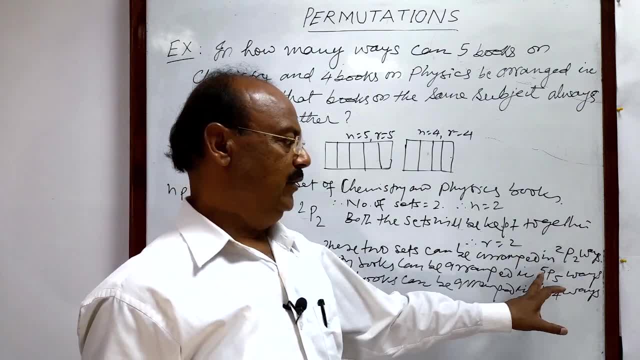 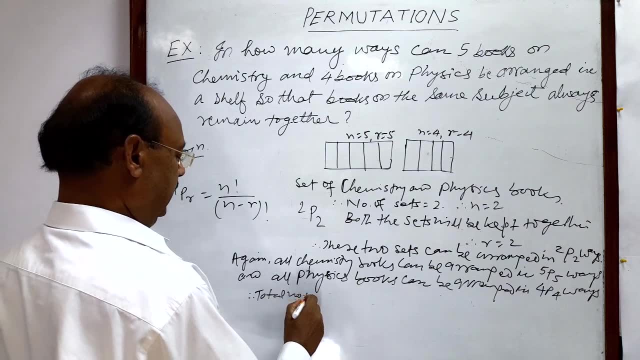 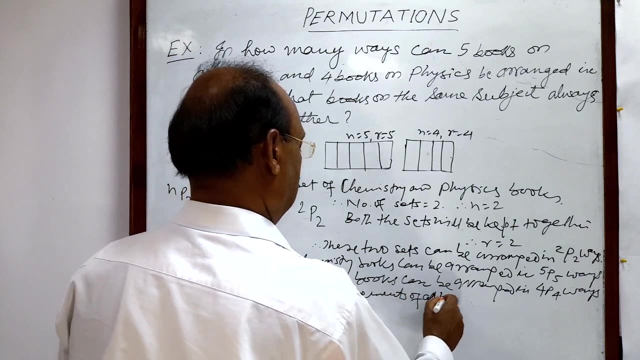 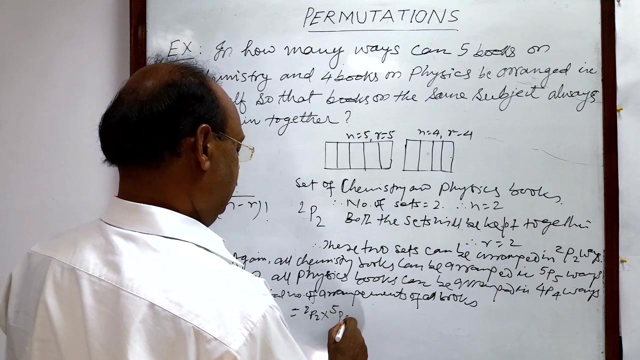 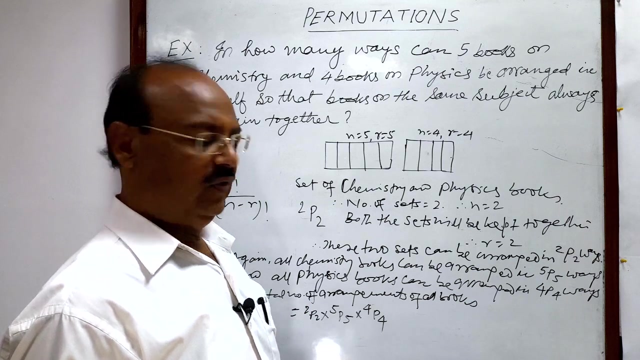 possible arrangements will be two p two into five p. five into four- p four. therefore, total number of arrangements of all books is equal to 2P2, 5P5 and 4P4.. After calculating it we will get the result. So 2P2 means this is: 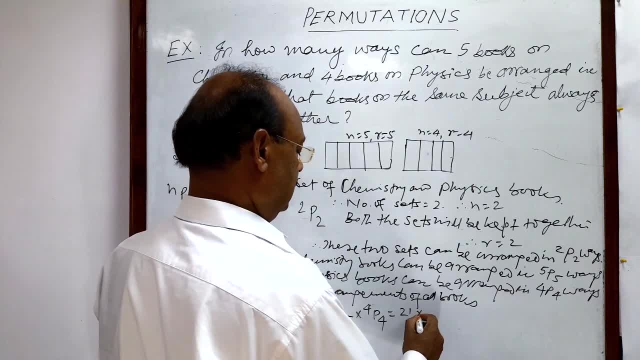 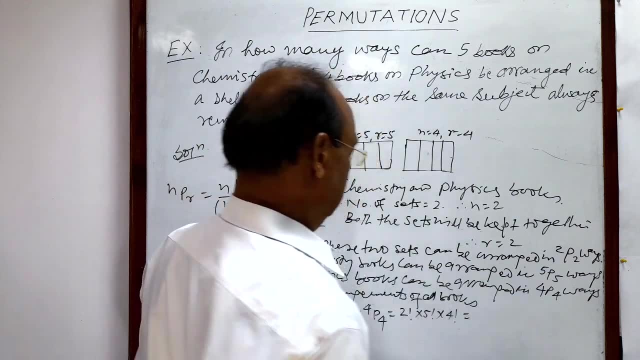 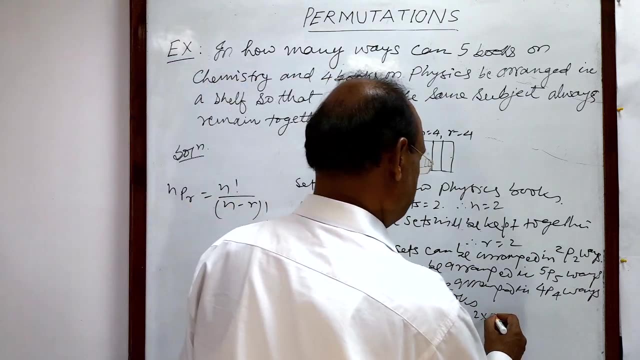 2 factorial. 5P5 means 5 factorial and 4P4 means 4 factorial. 2 factorial is 2, 5 factorial is 1 into 2, into 3, into 4, into 5, this is 120 and 4 factorial is 1 into 2, into 3 into. 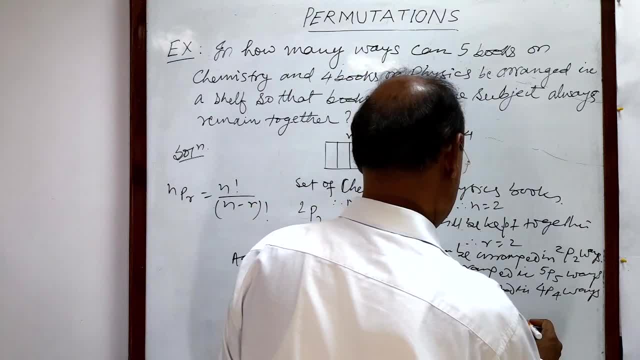 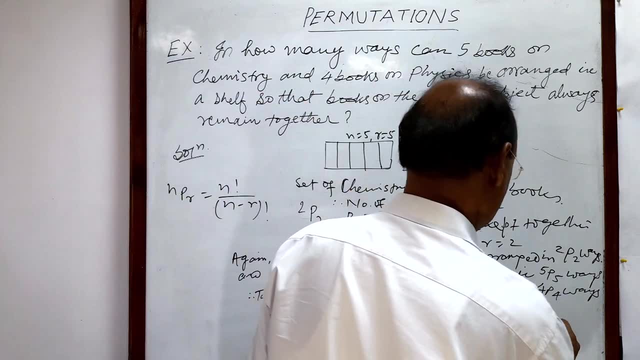 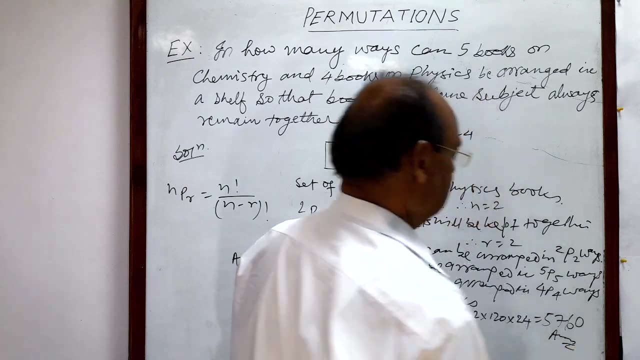 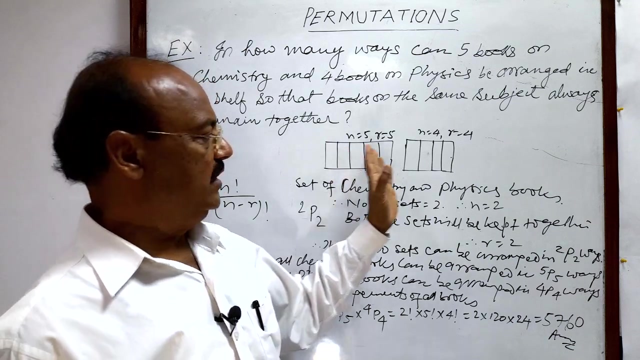 4 means 24. And whenever we multiply these numbers, we will get 576 and 0.. This is the answer: 5760 arrangements will be put in place. It is possible in this case, when 5 chemistry books and 4 physics books are arranged together. 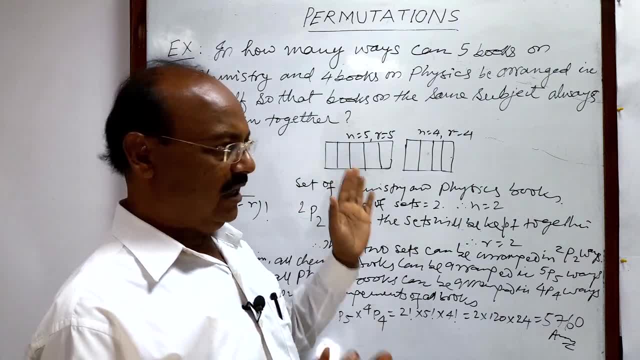 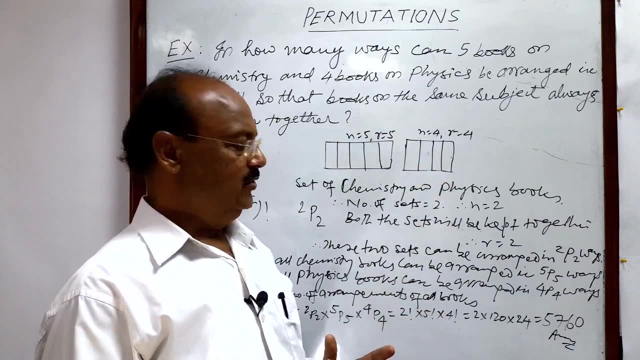 in such a way that all physics books are together, remain together, as well as chemistry books remain together. So this is the answer. Question is very interesting. Hope you have understood it.